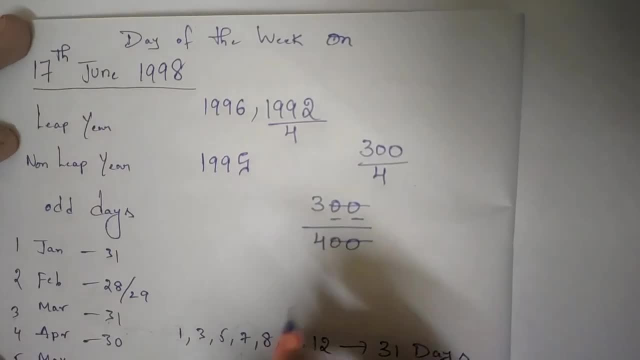 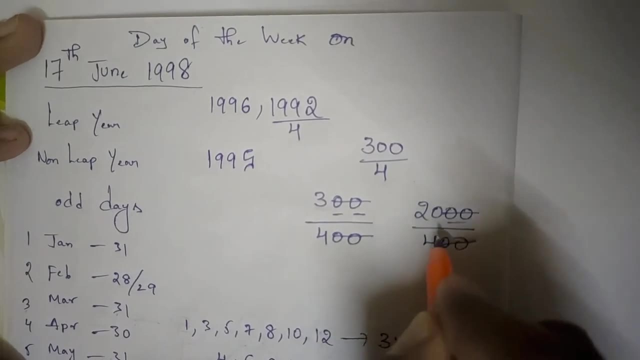 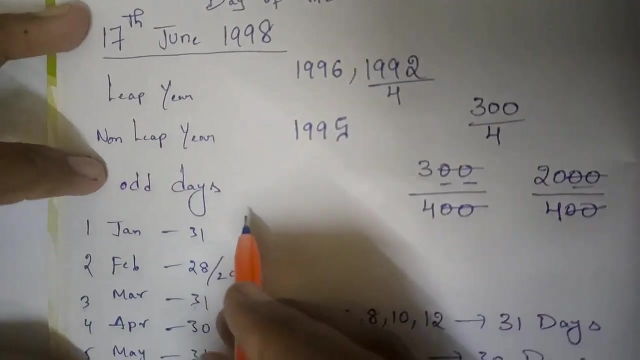 why it is not a leap year. if we are having any consecutive two zeros at the end of an year, then we need to divide by 400.. now 2000 is divisible by 4, then it is called a leap year. and what is this? odd days for a leap year. the number of days is equal to 366 and 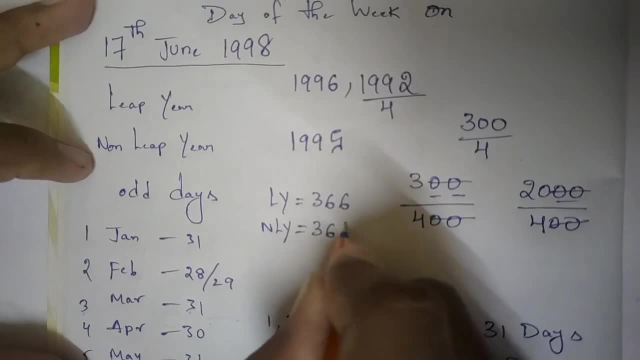 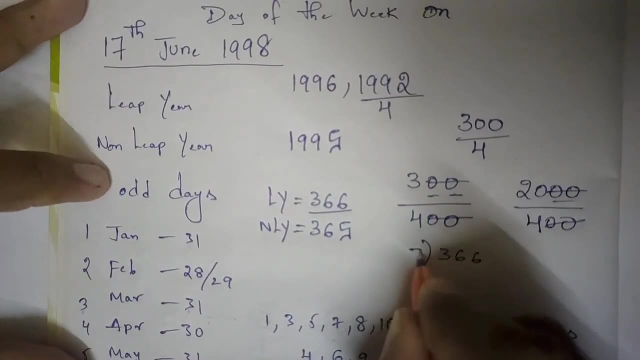 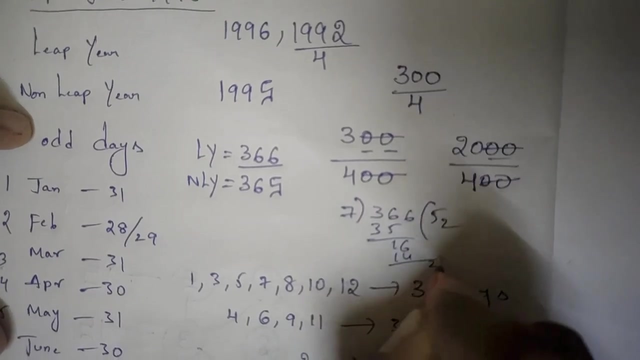 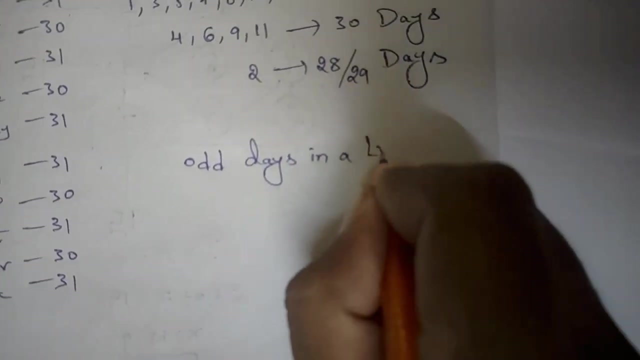 for non leap year. number of days equal to 365 odd days of. if we divide by 366 by 7, we get: 7 x 5 is 35.. 7 x 2 is 14.. We get 2.. Therefore, number of odd days in a leap year is 2.. 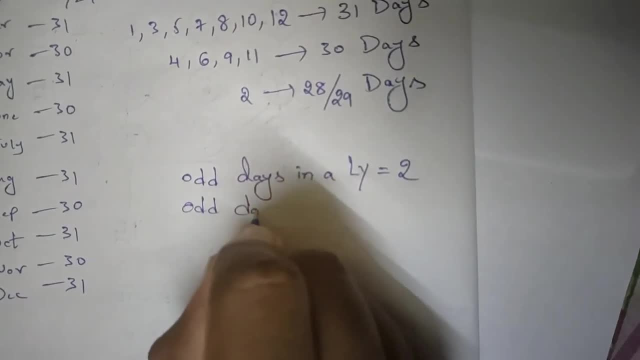 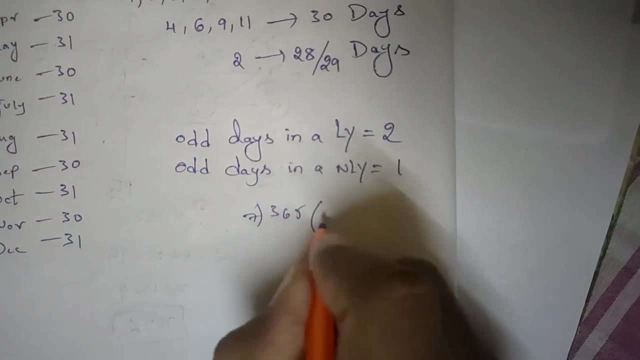 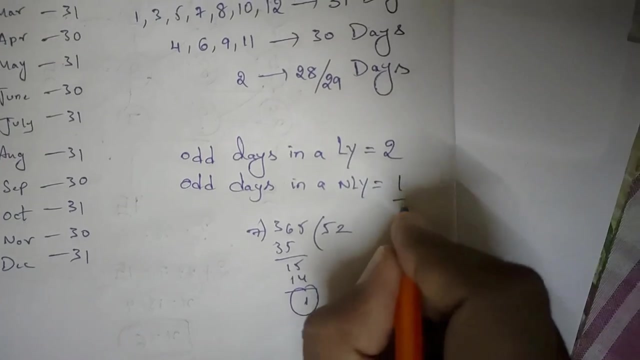 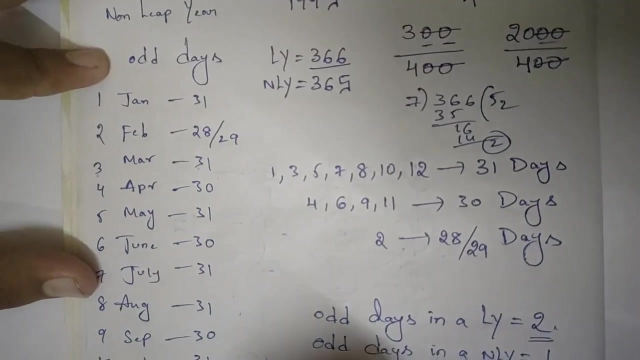 Odd days in a non-leap year equal to 1. 365 x 7.. Therefore, the number of odd days in a non-leap year is 1. And the number of odd days in a leap year is 2.. And we should have some basic idea about what are the months are having 31 days and which months are having 30 days. 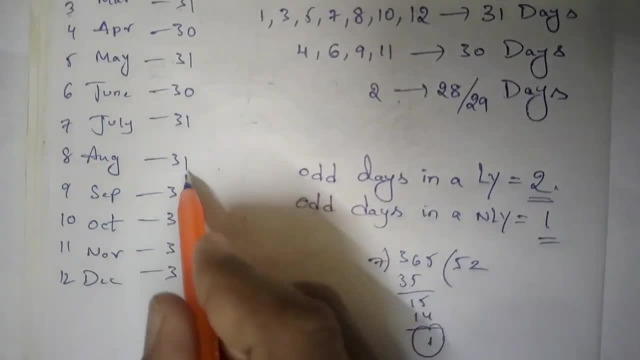 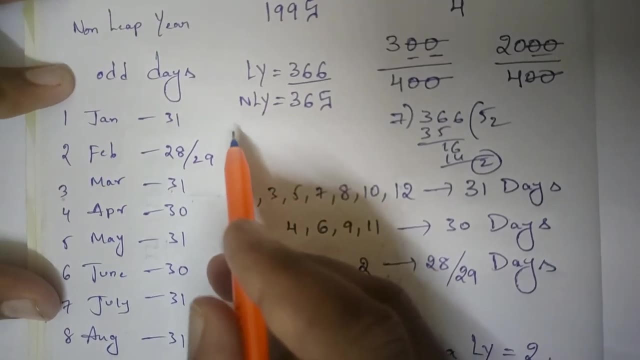 January, March, May, July, August, October, December. These months are having 31 days and February is having 28 days. for non-leap year and for leap year it is having 29 days And the remaining months are having 30 days. 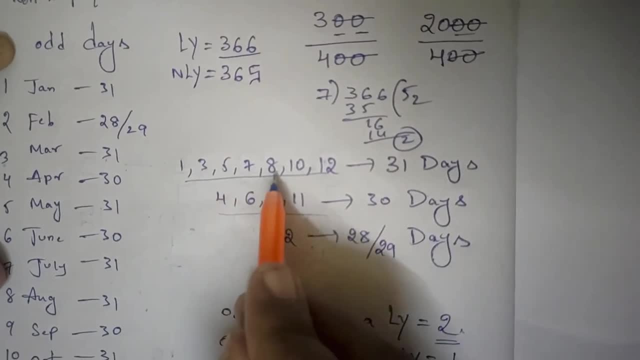 You can remember by using this code: 1,, 3,, 5,, 7,, 8,, 10,, 12.. These months are having 31 days, And 4,, 6,, 9,, 11.. These months are having 30 days. 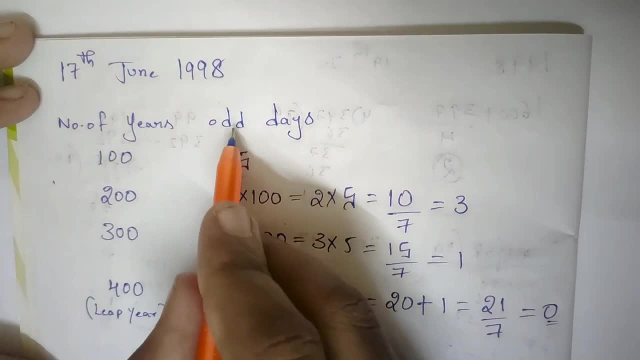 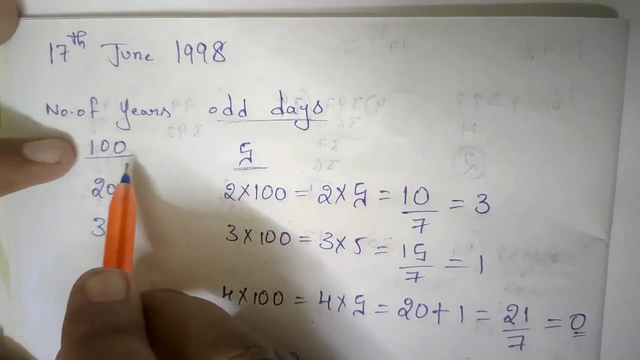 To solve this problem. we should have some more idea about the number of odd days For a period of 100 years. we are having 5 odd days. How I got these 5 odd days? To get these odd days, we need to calculate. 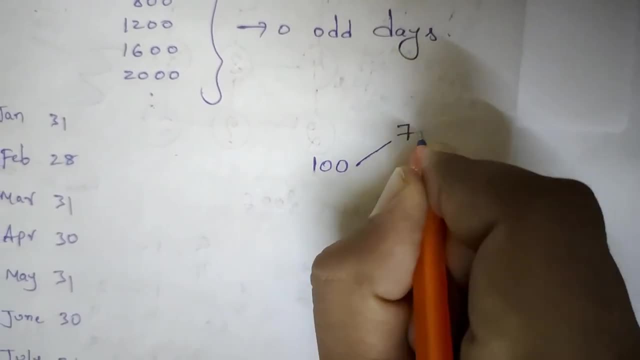 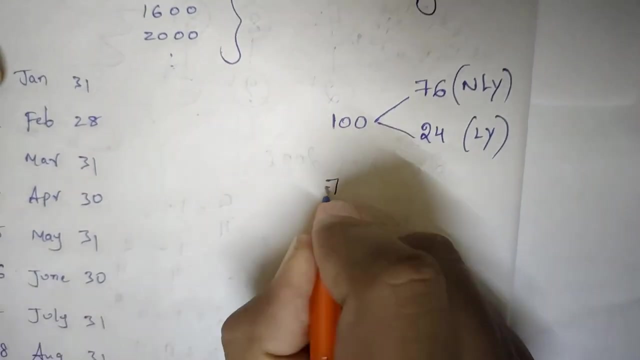 In a period of 100 years, we are having 76 non-leap years and 24 leap years- 76.. In a non-leap year, we are having only 1 day, 1 odd day. 76 x 1 equal to 76.. 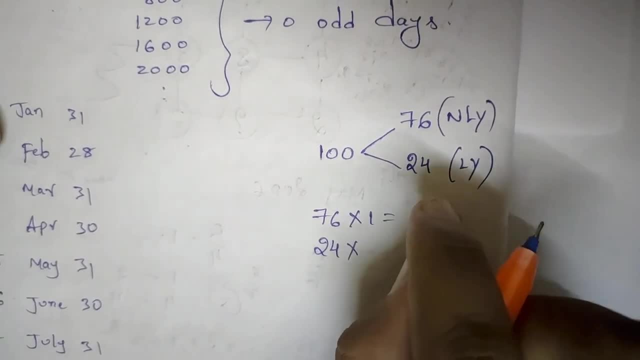 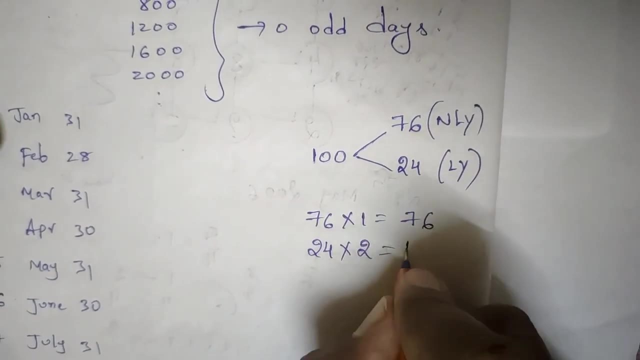 And in 20. And here we are having 24 leap years In a leap year. we are having 2 odd days. That's why here, 2. 24 x 2. 48.. Therefore equal to 124.. Now divide this 124 by 7.. 7 x 7 is 7. And 54.. 7 x 7 is 49. Therefore we got 5.. Therefore, the number of odd days in a period of 100 years is 5.. 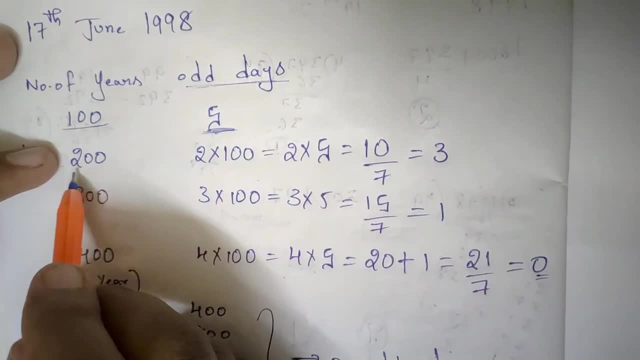 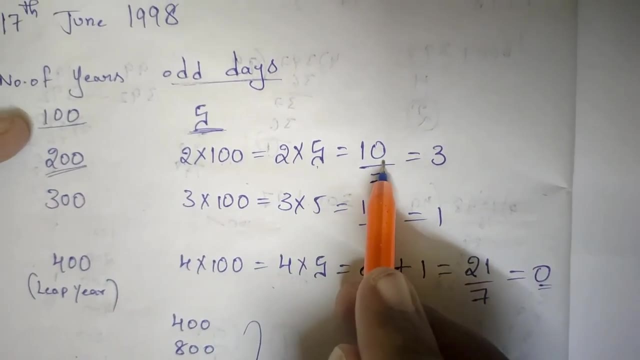 In the same way, number of odd days in 200 years is 2 x 100 years. For a period of 100 years we are having 5 odd days, 10.. Now divide this 10 by 7. We are getting remainder 3.. 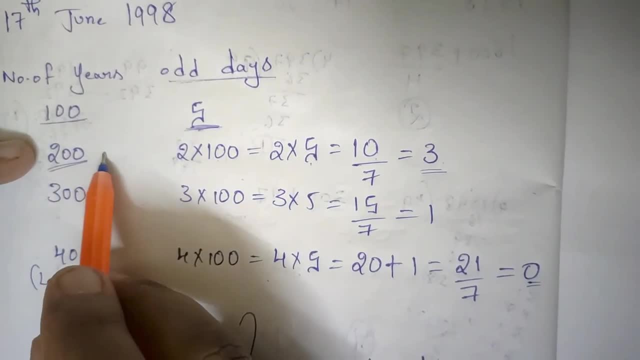 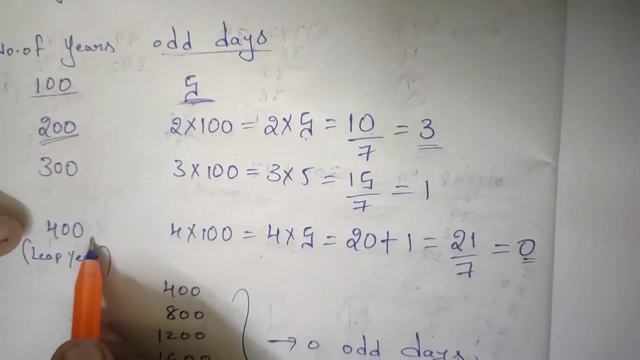 Therefore, number of odd days equal to 3 in a period of 200 years. In the same way, for 300 years we are getting 1 odd day For 400.. For 400, it is somewhat special, Like 4 x 100.. 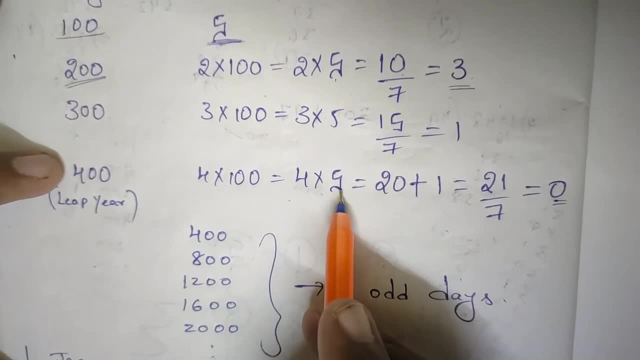 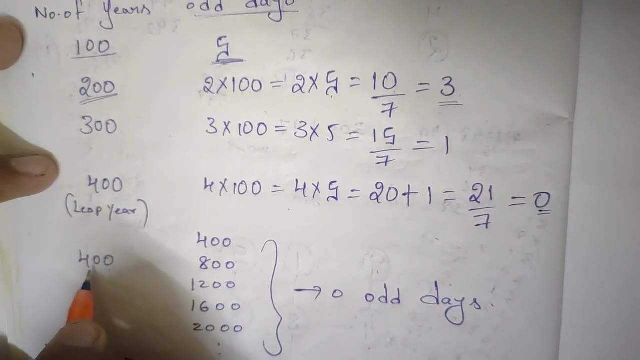 For a period of 100 years, we are having 5 odd days. 4 x 5 equal to 20.. Now this 400 is also a leap year, Because 400.. Now here we are having 2 consecutive 0s at the end. 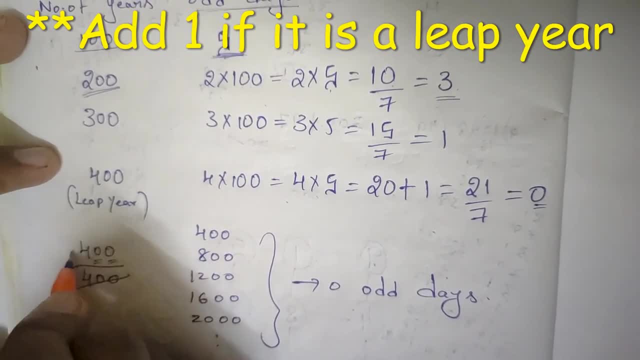 That's why we need to divisible by 400.. Now, this is divisible by 400.. That's why it is also a leap year. For a leap year, we are having 1 odd day Plus 1., Equal to 21.. 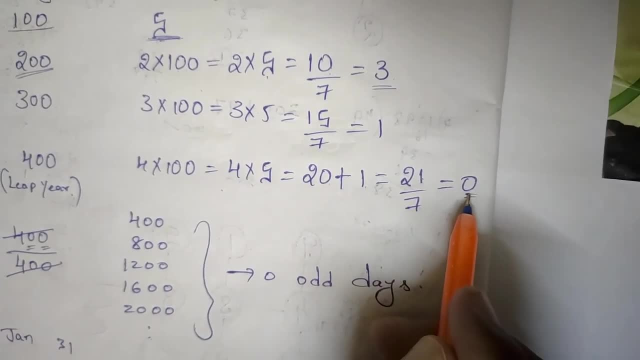 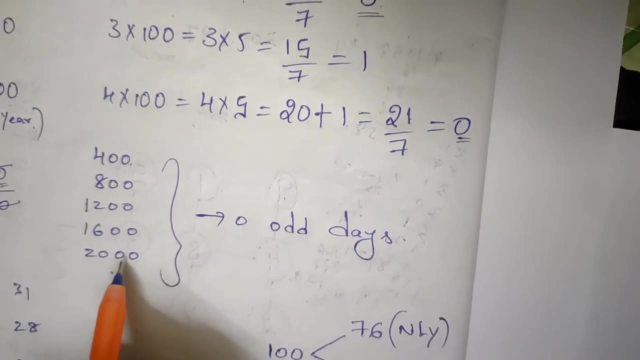 Now divide this 21 by 7. Now we are getting 0 odd days For 400.. In the same way for 400. 800. 1200. 1600. 2000.. The number of odd days are 0.. 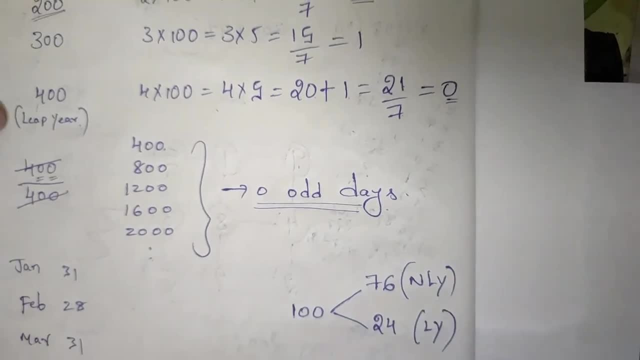 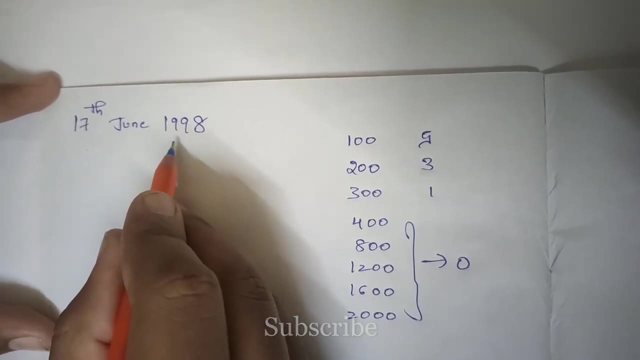 We should follow this method to solve this problem. Now we are going to solve this problem. 17th June 1998.. Here we have to take the year before than this, 1997.. Because still, 1998 is going on. 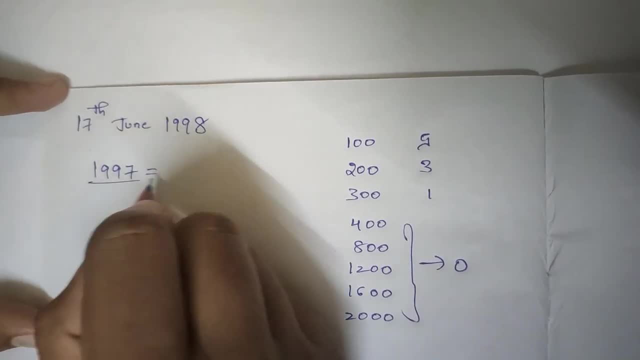 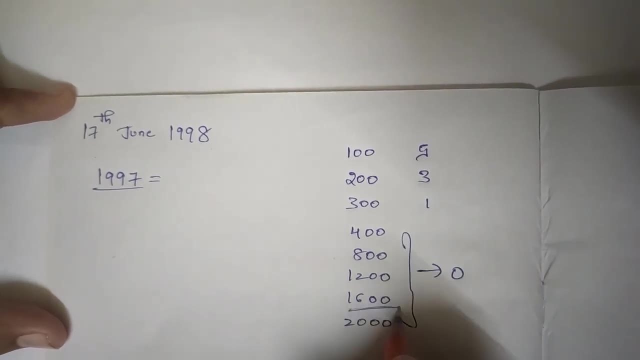 Now we have to expand this 1997.. In such a way that this is nearer to this number of odd days equal to 0.. We need to take the nearest one. I am taking 1600.. 1600 plus 300 plus 97.. 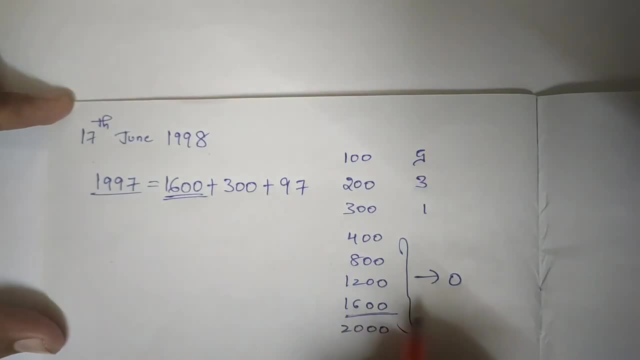 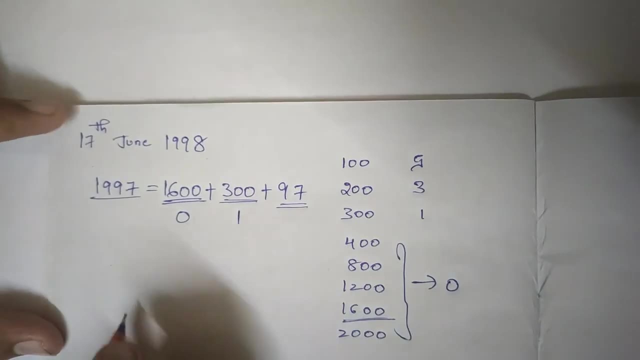 The number of odd days in 1600 is 0.. The number of odd days in 300 is 1.. And we need to find the number of odd days: 97.. First of all, we need to find the number of leap and the number of non-leap years in 97 years. 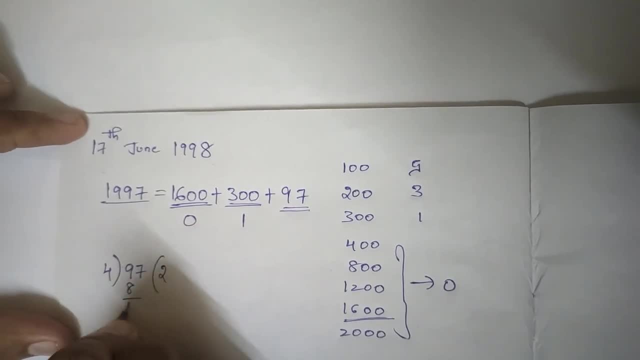 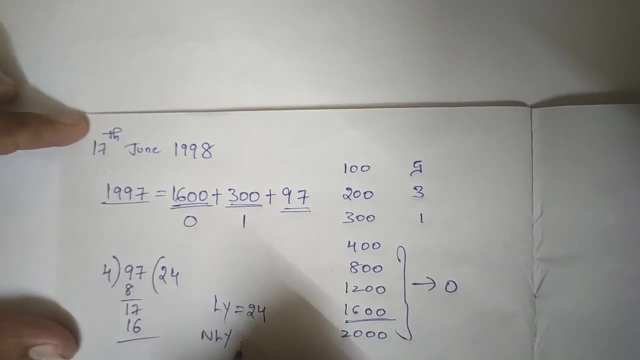 4.. For 2 is 8.. For 4 is 7.. For 4 is 16.. The number of leap years is 24.. And the number of non-leap years equal to 97 minus 24, which is 73.. 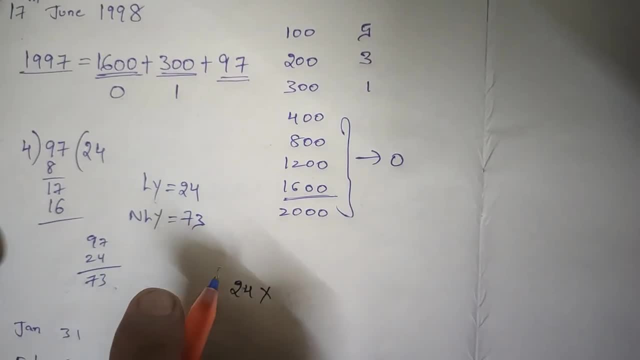 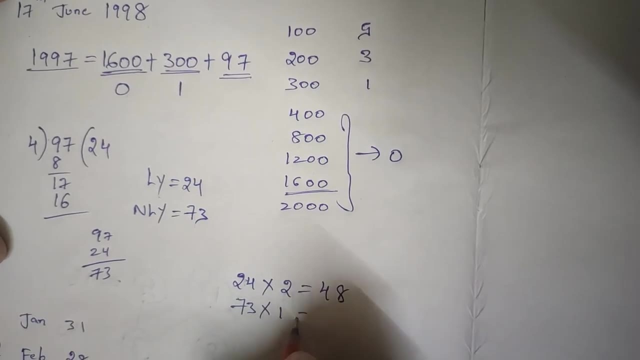 24.. Here there are 24 leap years. For a leap year, the number of odd days is 2.. Therefore 48.. For a non-leap year, the number of odd days is 1.. 73 into 1, equal to 71.. 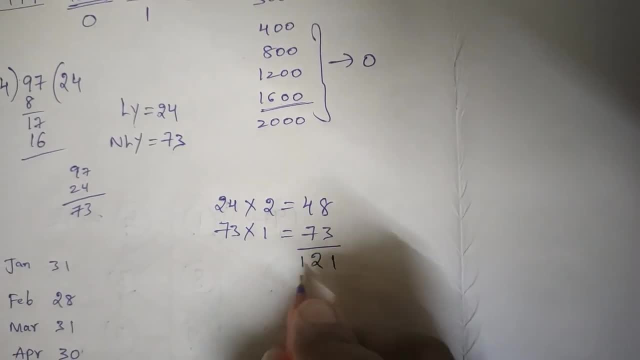 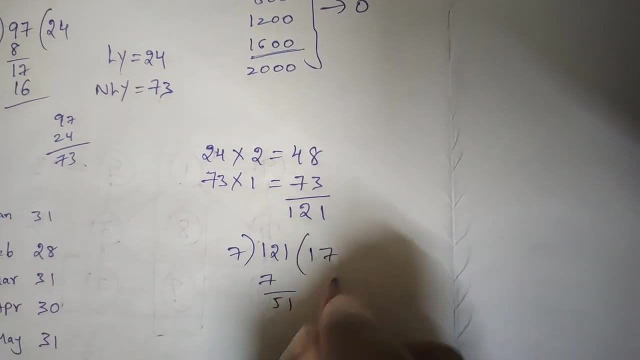 Total number of days equal to 121.. Now We need to divide this 121 by 7.. 7 times 7 is 7.. 7 times 7 is 49.. The number of odd days equal to 2.. For 97,, the number of odd days equal to 2.. 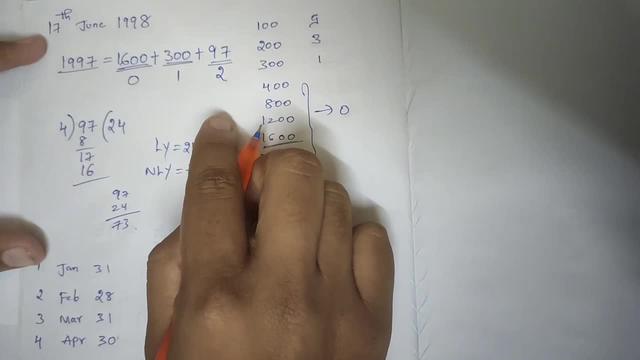 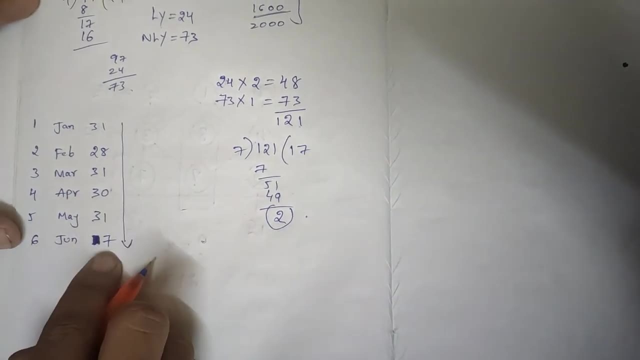 97 years Now. still the problem is not completed. We need to find till 17th June. Now we need to add till June 17th 31 plus 28.. Because this 1998 is not a leap year. 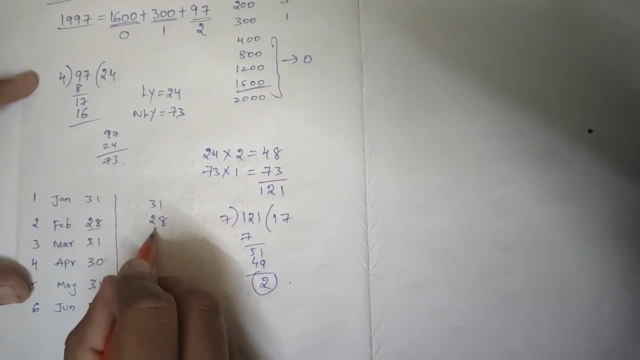 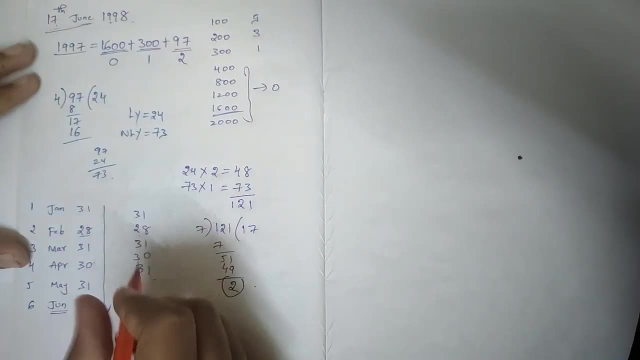 That's why we need to take only 28.. 31,, 30 and 31. June. Still we need to find June 17th. That's why 17. Only 17. Now we get 1 plus 10.. 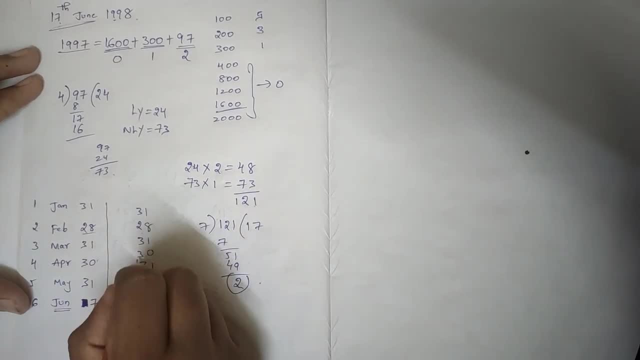 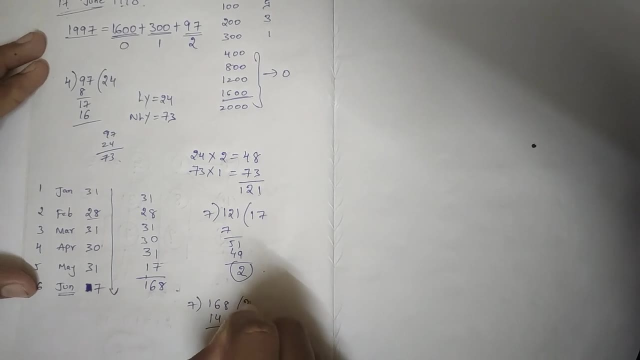 18. 168.. Now divide 168 by 7.. 7 times 2 is 14. 28.. 7 times 4 is 28.. Now we get 0. That means there are no odd days. 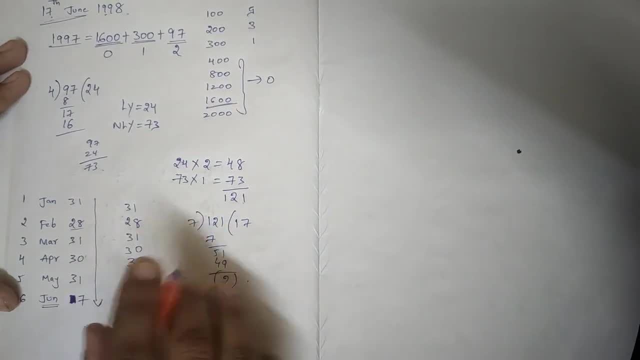 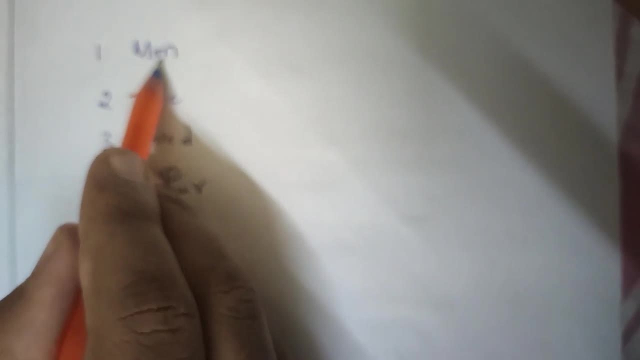 From January 1 to June 17th. Therefore, 0 plus 1 plus 2, equal to 3.. But what is this 3?? Monday, Tuesday, Wednesday, Thursday, Friday, Saturday, Sunday. Our task is to find the day of the week.